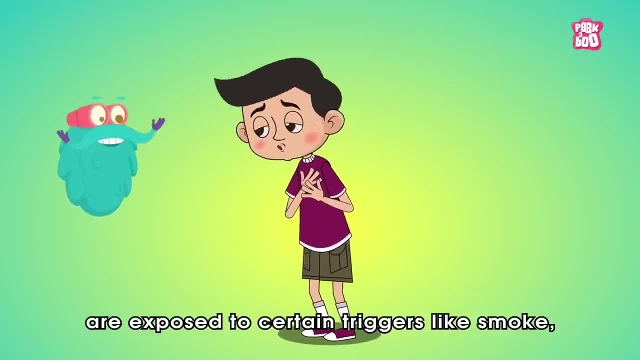 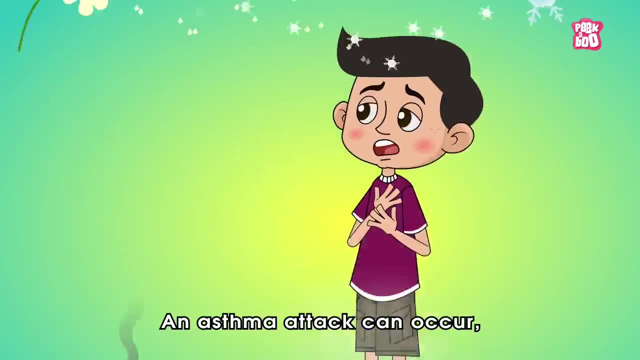 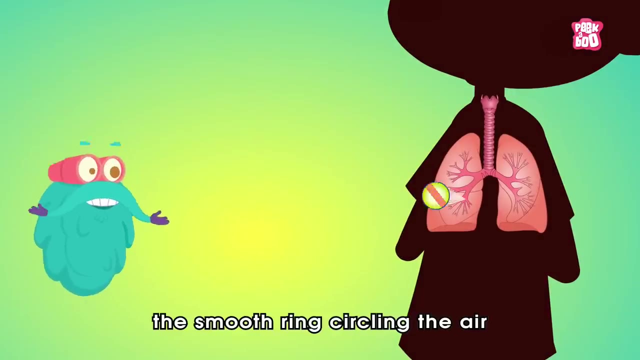 But when people with asthma are exposed to certain triggers like smoke, dust, pollen, colder climates, etc. an asthma attack can occur, making it difficult for them to breathe. And that is because the smooth ring circling the air passages in the lungs tightens and narrows down. 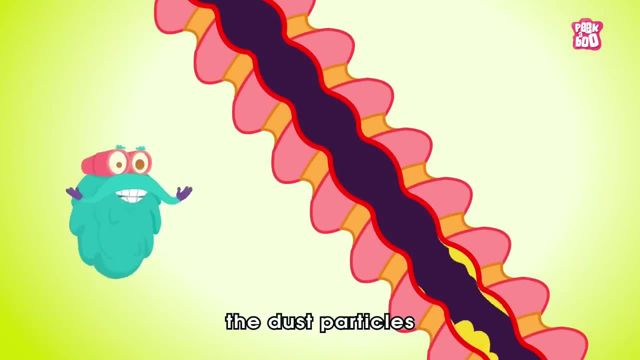 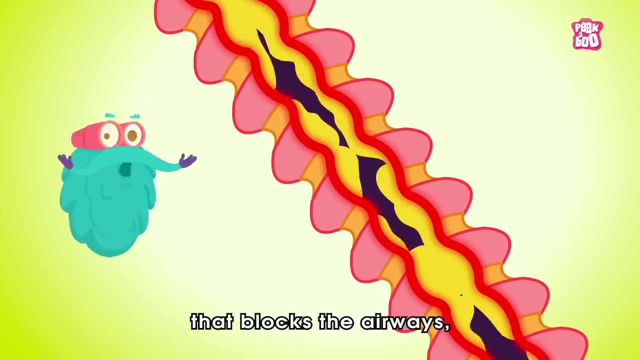 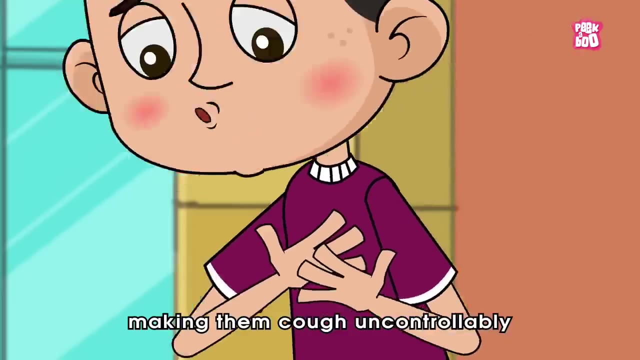 And, at the same time, the dust particles cause the mucosal lining to swell and produce lots of thick mucus that blocks the airways, making it harder for the infected person to breathe As they feel their chest tighten, making them cough uncontrollably due to swollen airways. 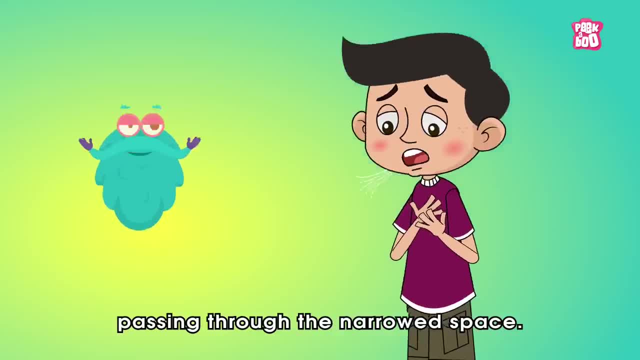 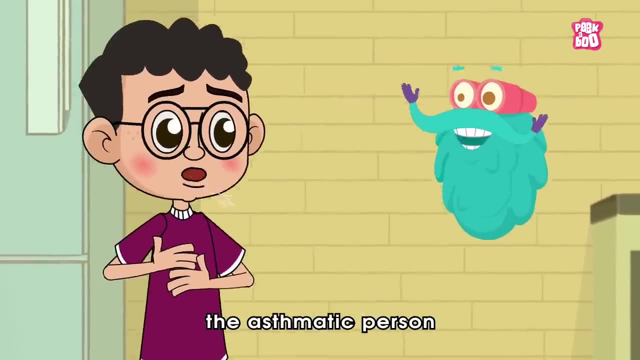 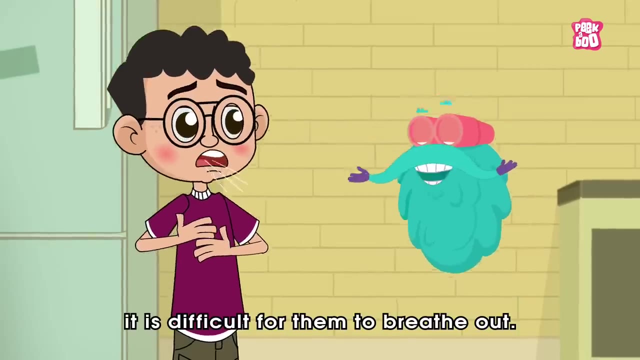 they make a wheezing sound as the air whistles while passing through the narrowed space. These symptoms may seem like the asthmatic person is having difficulty in breathing in, But in reality, during the attack, it is difficult for them to breathe out. 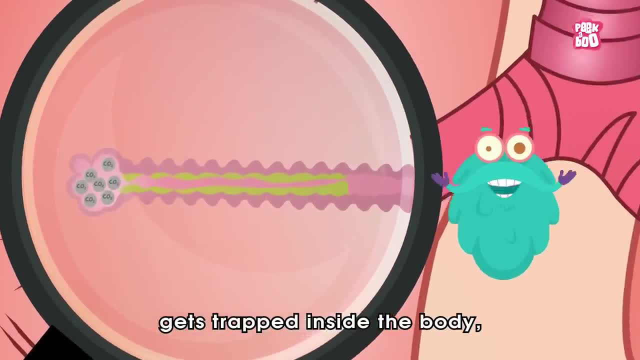 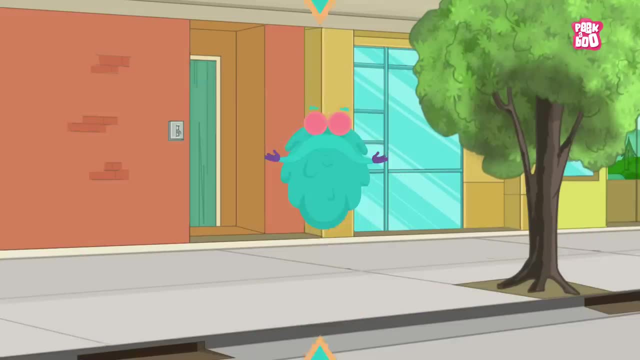 That's because carbon dioxide gets trapped inside the body, cutting the supply of fresh oxygen, resulting in an asthma attack. But the crucial question is: how can we prevent these attacks? Well, one way to limit asthma includes knowing what triggers it and avoiding them. 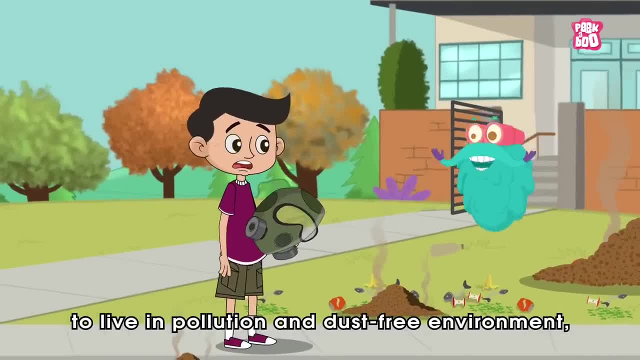 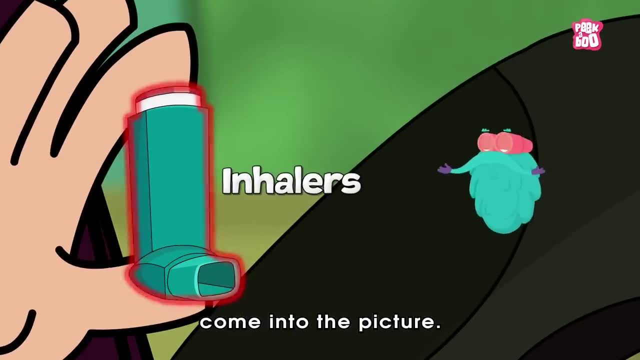 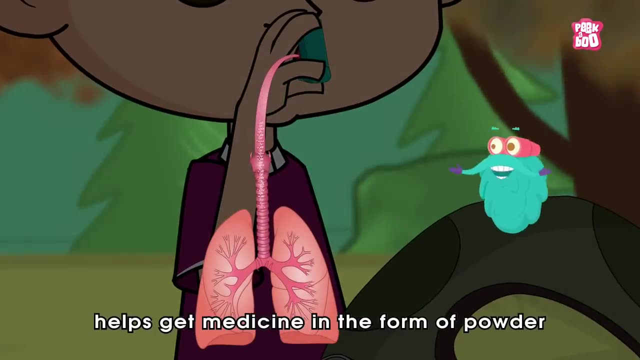 But unfortunately it isn't really possible to live in pollution and dust-free environment. So this is where inhalers come into the picture. Most asthma medicines need to be breathed in, and an inhaler helps get medicine in the form of powder into the lungs. 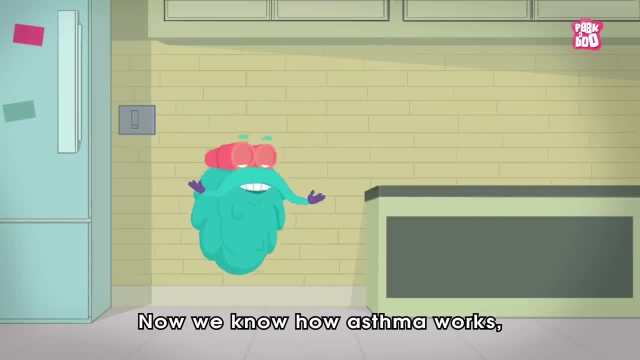 Now we know how asthma works, But the most important question is: what causes it? Well, on an honest note, we don't know. Yes, no one really knows the reasons behind its cause, Although it is believed that certain genetic and environmental factors could be the main cause.